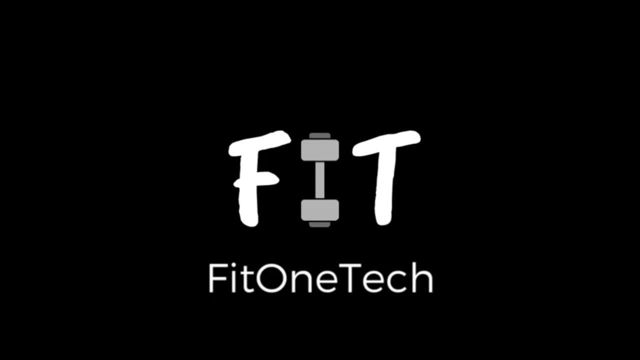 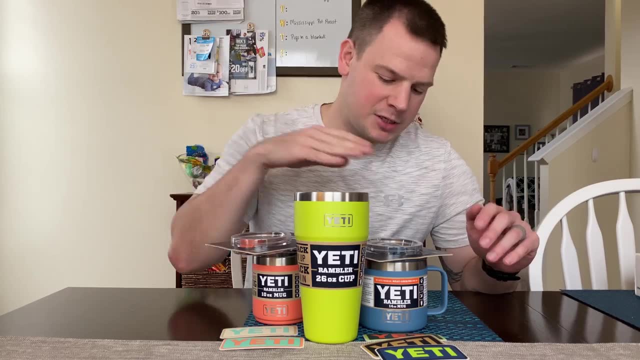 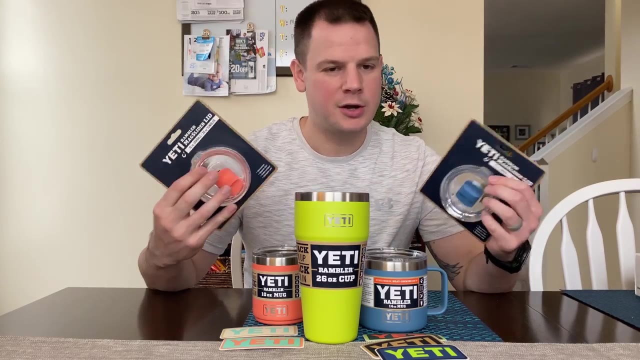 What's up guys? Aaron's here, It is 2020.. The mailman just came ordered these. got the new colors that came out. Pretty big fan of them. I kind of like bright colors. I do have a lot of steel products- darker colors, Obviously, being in the military, I kind of. 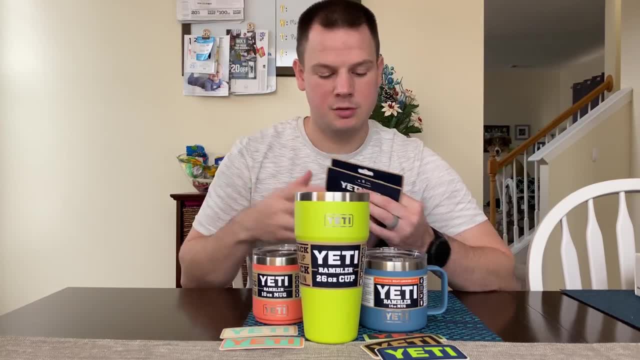 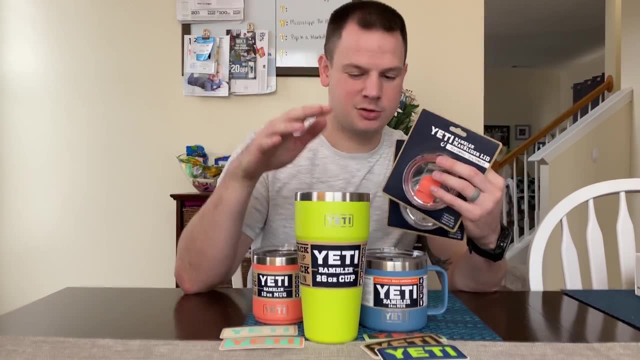 bring stuff. I kind of was looking for a new cup, so that's kind of what got me onto this. But you see the new colors. We got the new mag lib colors, Cool. So we're going to check out the Pacific Blue, the Coral and the Charteroose- Charteroose bright yellow in. 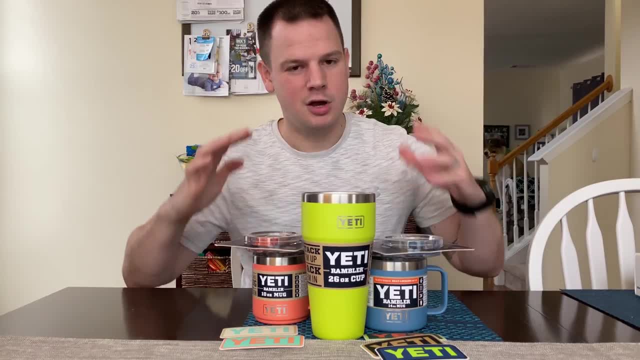 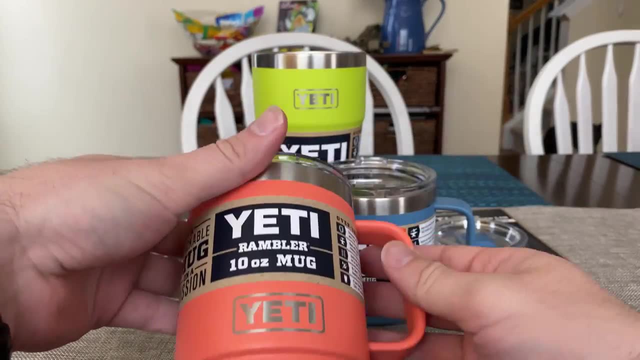 your face. We're going to take a look at those. Hey, if you guys really enjoy the channel, be sure to like, hit subscribe, and I'm not going to get too long in the intro, We'll get right into it. So let's get a little more. just take a quick look Again now. this is 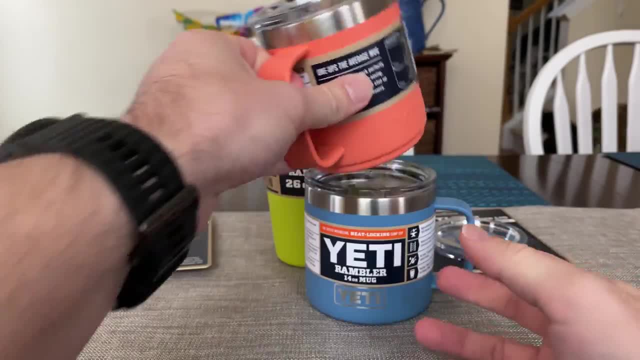 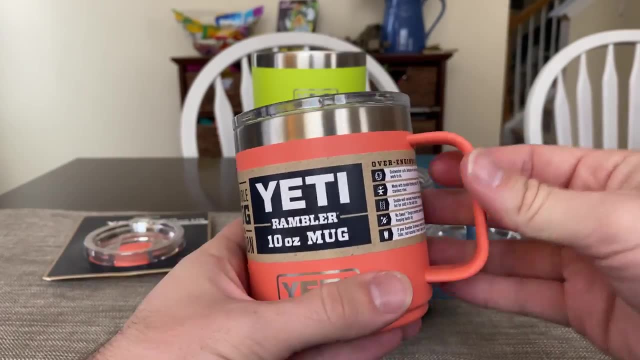 the 10-ounce. These are pretty new. These are the stackables. Obviously it doesn't stack with the larger one. It kind of does, but if I had two I can kind of demonstrate it. But I really like this color. You know, even in the 40s it's kind of like you know. 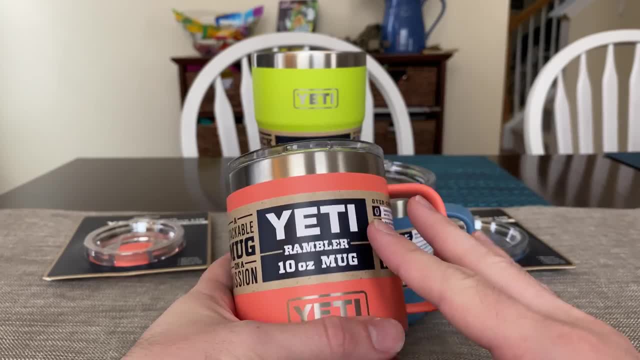 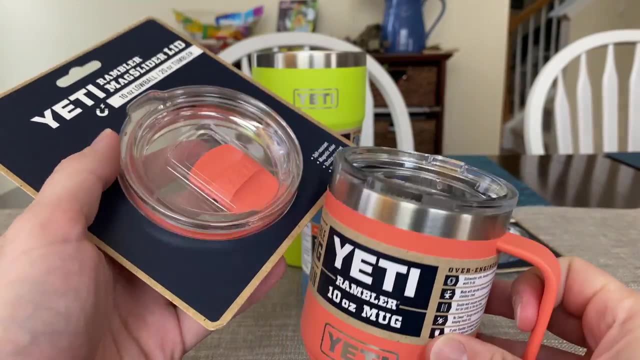 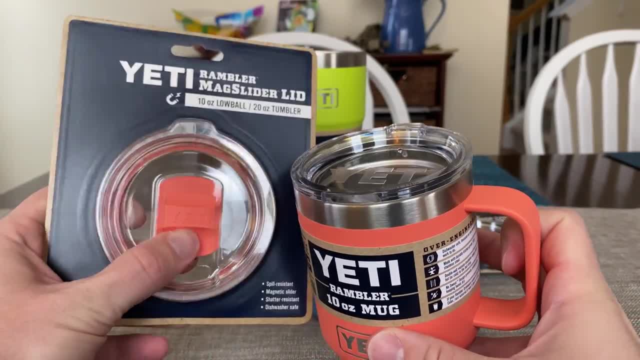 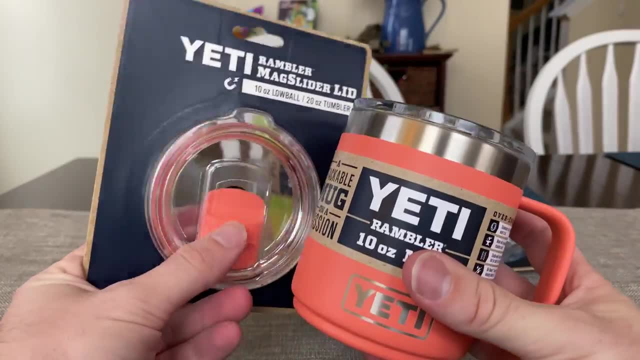 on the iPhone 11 Pro Max, but it's definitely looks a little more orange. It's definitely pinkish in person, It's just getting washed out a little bit. Maybe I can try to color correct that, But yeah, so these lids only fit these 10-ounce ones and the regular lids. 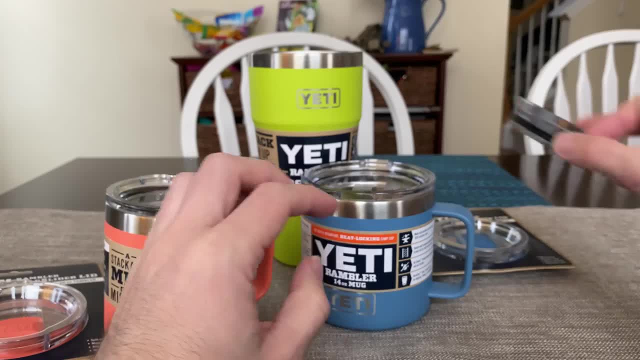 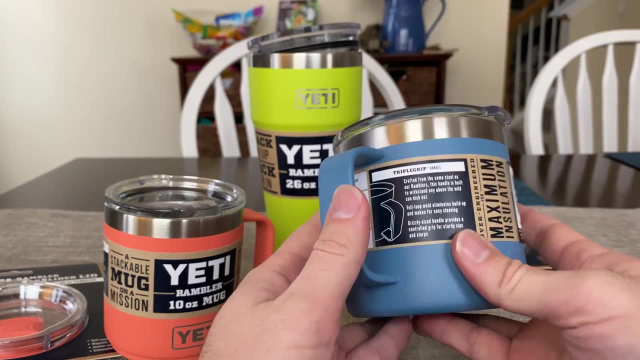 they don't fit. Actually, this big cup, it's actually going to take the large one up here, something on here. But we'll take a look at the blue. The blue, based off what I'm seeing, it looks very similar. The color is very accurate. here Again, you see the retail prices here: $24.99,. 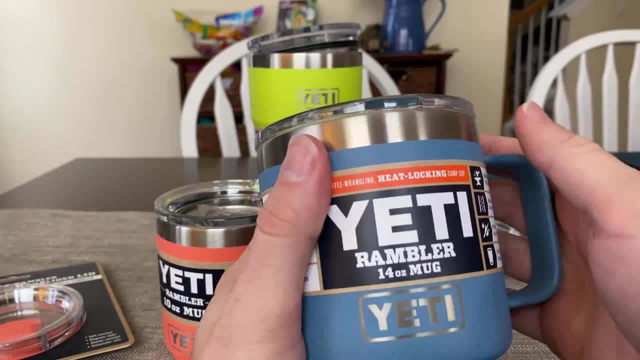 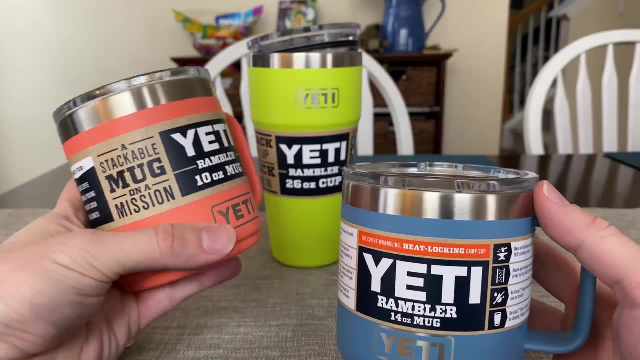 $24.99.. So it's just size My wife uses. she has one of these in that green color, that light green, kind of turquoise color- I can't remember the proper name of it right now, Whatever, But yeah. so she really uses her mugs a lot And I'm going to show you guys. 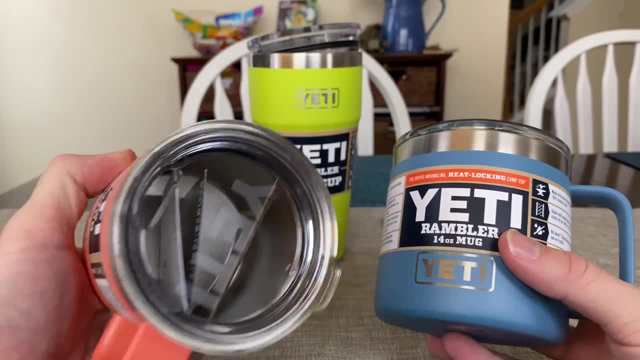 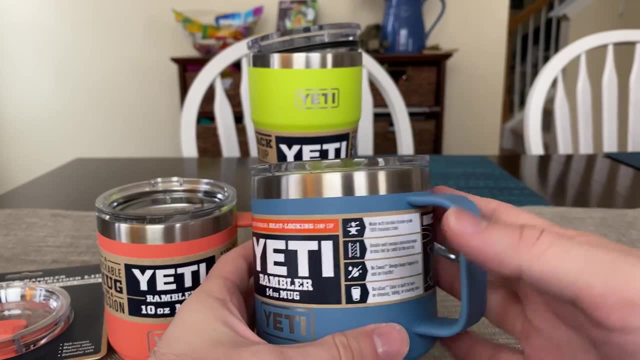 what I got. So I got her kind of the smaller one which actually feels really nice in the hands. It does really feel good. May order one of myself. I use the Hot Shot mainly for coffee or the Rambler cups, So never been a big fan of this big mug, but I could see. 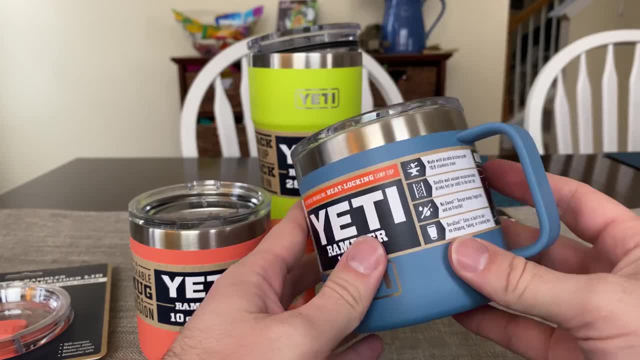 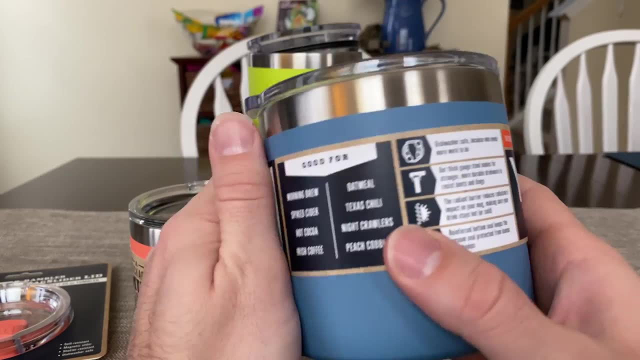 my wife using this one a lot more. She's going to be coming home and using it soon, But yeah. so here's the blue Cool. See what it's good for. You know peach cobbler, Yum, So okay. 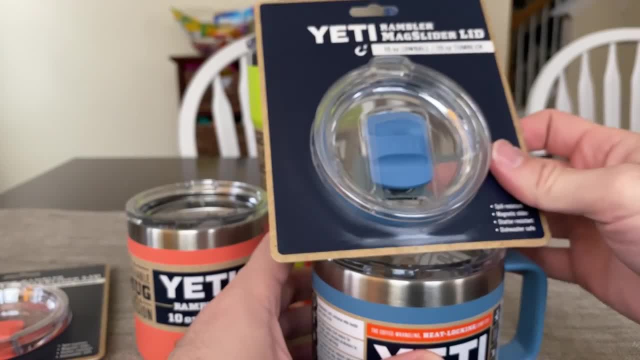 But yeah, so there's that. And again, I'm going to show you guys what I got. So I got this one right here. I'm going to show you guys what I got, So I got this one right here. And again, this one doesn't directly fit, but she can alternate between this or on the. 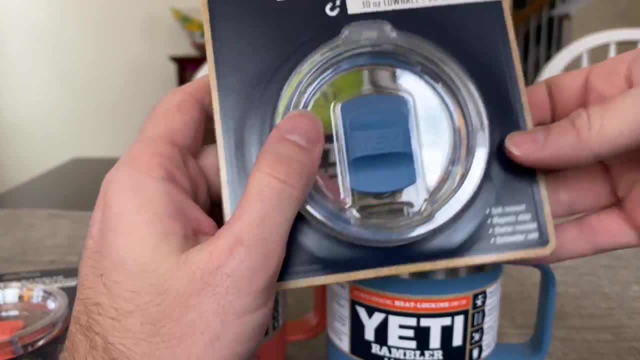 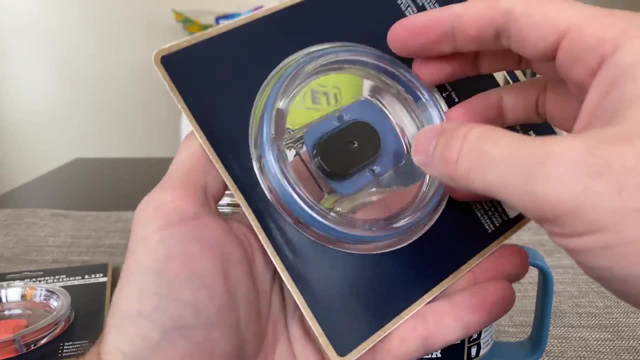 Ramblers that we have. We got a couple of different colors of Ramblers. So yeah, So that's the Mag Slider lid. Again, the big difference is the color of the Mag Slider, And then you see the actual seal. The gasket itself is of these colors too, So it's kind. 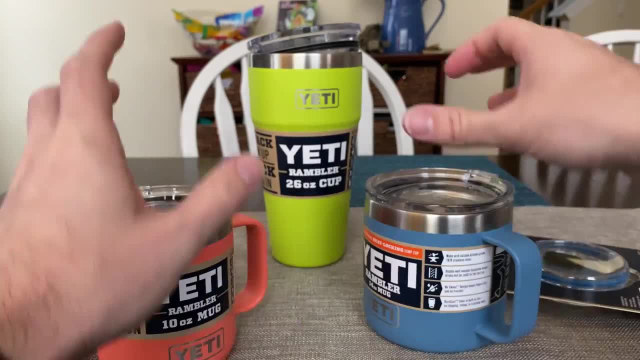 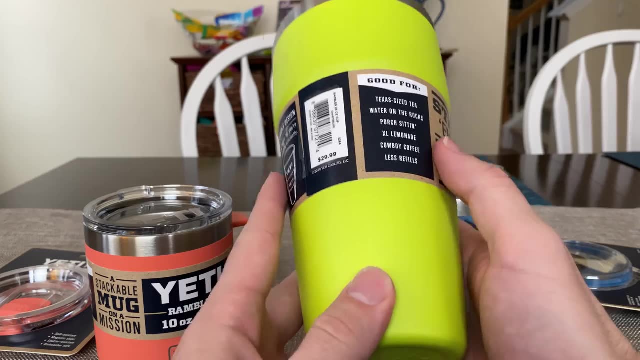 of nice of how those look. And then, of course, we got the very bright yellow. I hope I'm saying this right, Chatteroos. And this is the stackable 26 ounce cup, Now again $29.99.. So that's what they recommend it for. This is going to be my cup. that's kind of just. 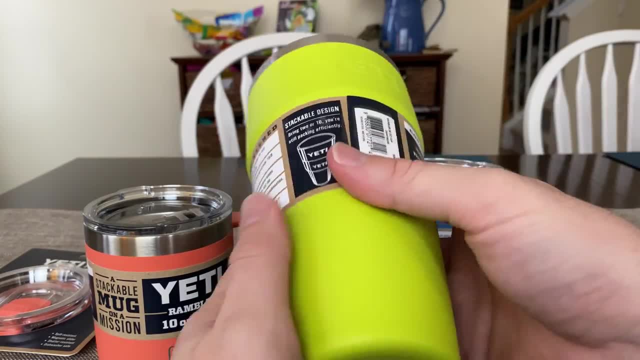 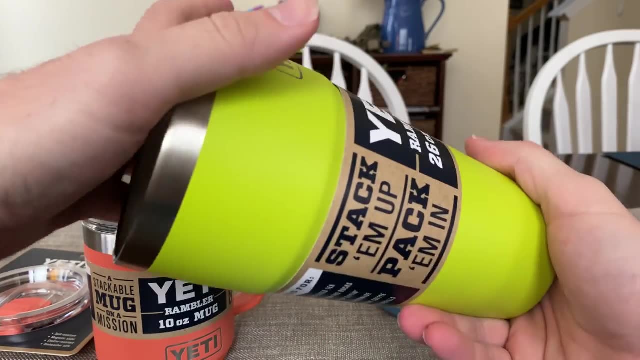 fit. you know, regular like lemonade, not really water. I have water cups. I got water, you know, 64 ounce, the the Rambler big one, not the half gallon, but not the new design. So that's kind of what I use them for. So it's nice to just kind of have a cup in my 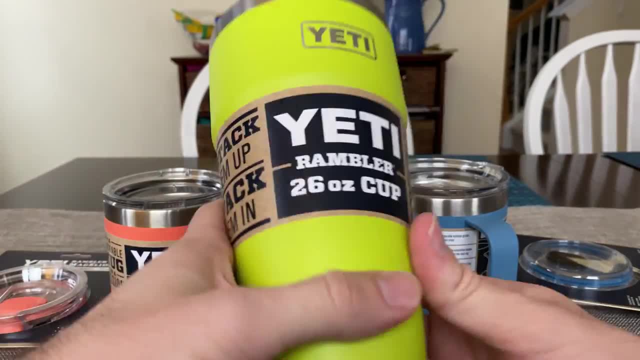 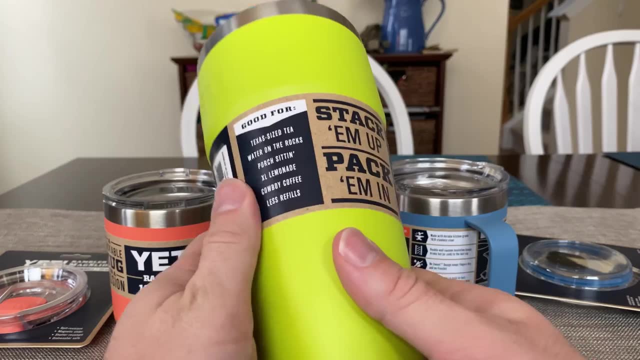 bag that I can just throw stuff in, maybe mix protein, whatever you know right, Keep stuff cold, Then I'm not going to just use just for water. So there's that, This color very accurate to what you're seeing right here. 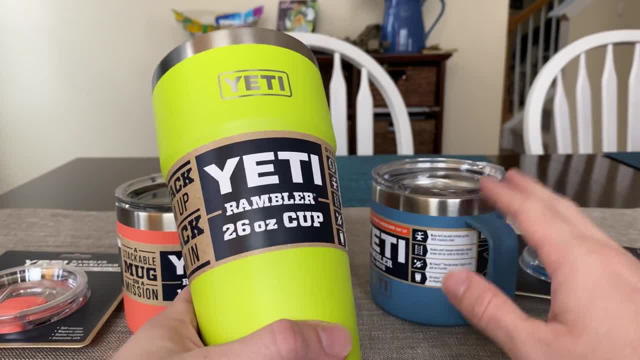 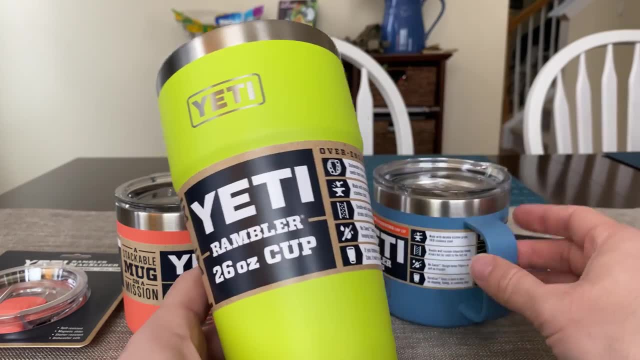 Again, this one's kind of a little washed out, pretty accurate, pretty accurate of what you're going to see. Honestly, like wasn't a fan when they first came out, but seeing them in person they're really nice. I really do enjoy them. The blue is really nice, It's. 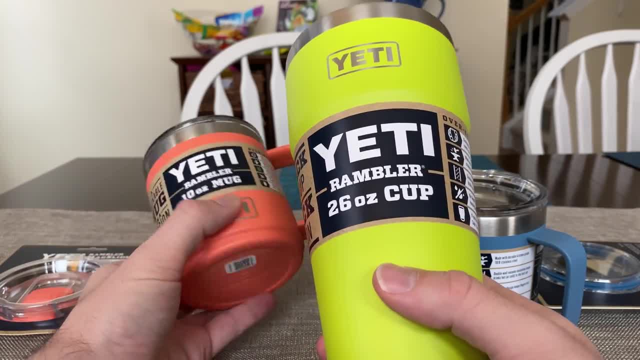 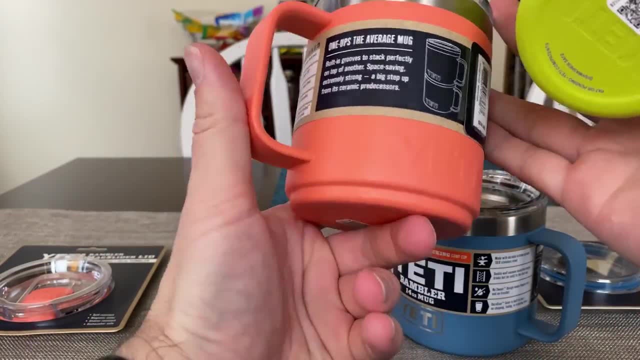 a little more UNC blue- not UK blue, whatever- But this pink color actually looks really good. This, the coral, looks really good in person, So it's a good color that came back out with. my dog really wants to come outside, But I'm a big fan of this. I'm going to get.